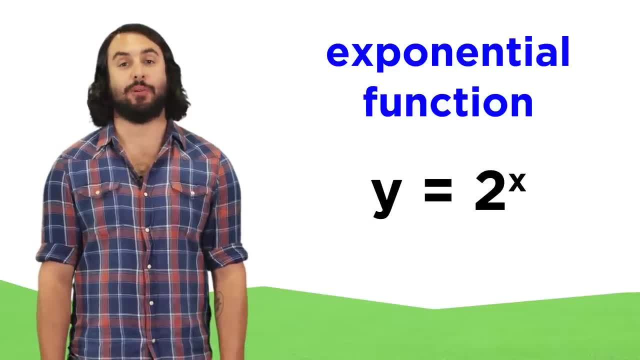 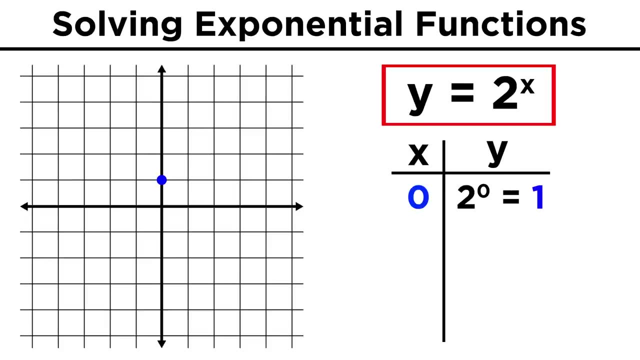 This would be called an exponential function, because a variable is acting as an exponent. To see what these do, let's plot a few points. When X is zero, Y is one, because anything to the zero power is equal to one which we 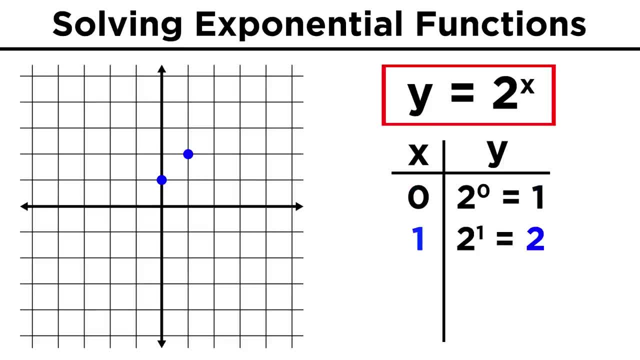 learned when we went over the rules of exponents. When X is one, Y is two, because two to the one is two. When X is two, Y is four, because two squared is four. When X is three, Y is four. 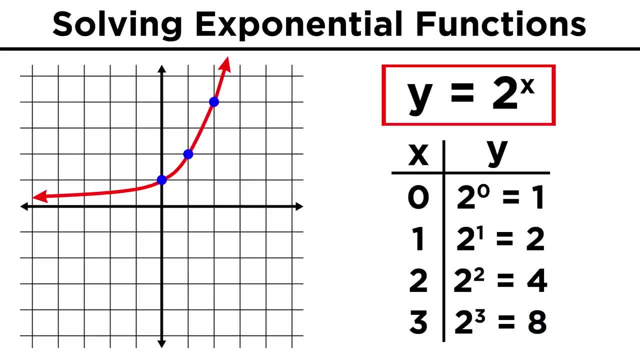 When Y is eight and so forth. As we can see, the function grows very rapidly as X increases. This number that is raised to the exponent is called the base, and changing the base will produce different exponential functions. We could have ten to the X, which will increase by an order of magnitude every time X increases. 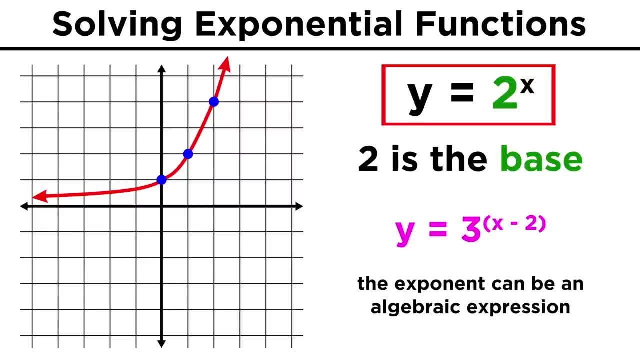 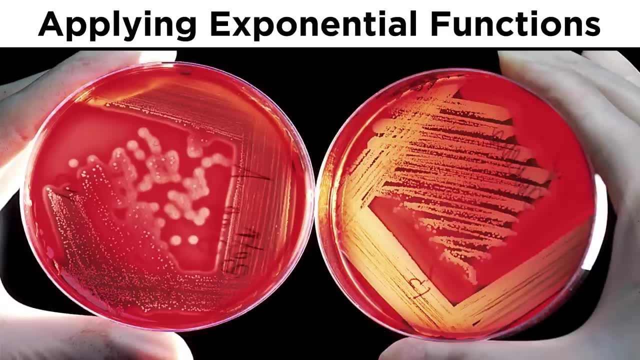 by one. The exponent can also be an expression like with three to the quantity X minus two. The only parameter is that the base must be positive and not equal to one. Exponential functions are valuable because they can model a number of real-world situations. 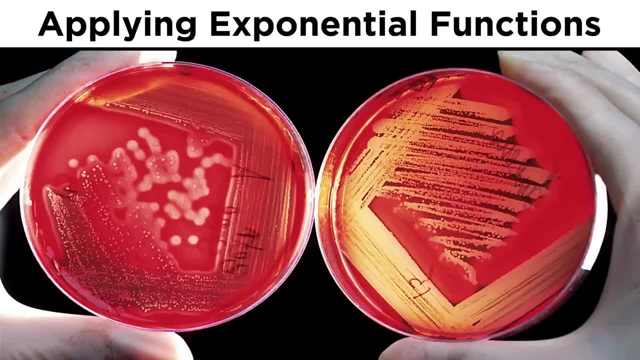 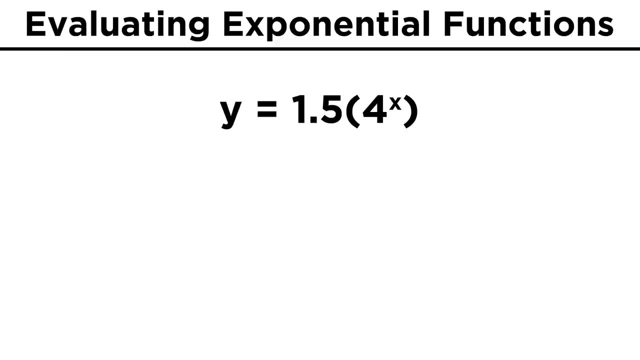 where rapid increase or decrease occurs. Population growth can often be modeled by an exponential function, especially for something like bacterial cultures or the spread of diseases. They are easy to evaluate on your calculator. One point five times four to the X. if we want to evaluate this for X equals three. 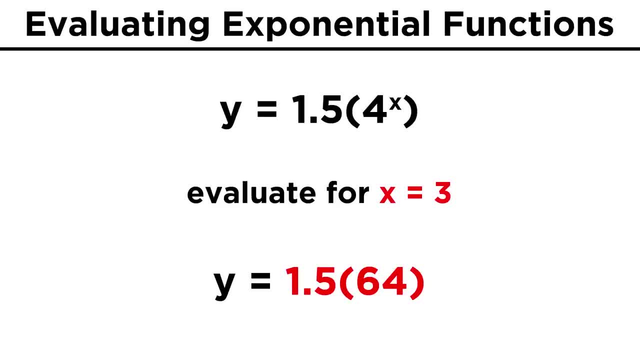 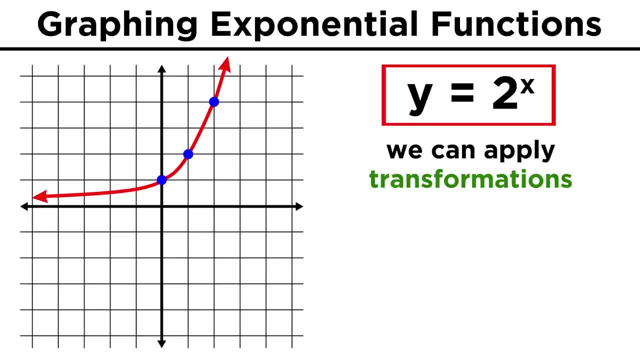 we just cube four to get sixty-four and then multiply by one point five to get ninety-six. Graphing can be a little trickier, but as long as we know what the basics look like, we can apply transformations just like we did for parabolas. 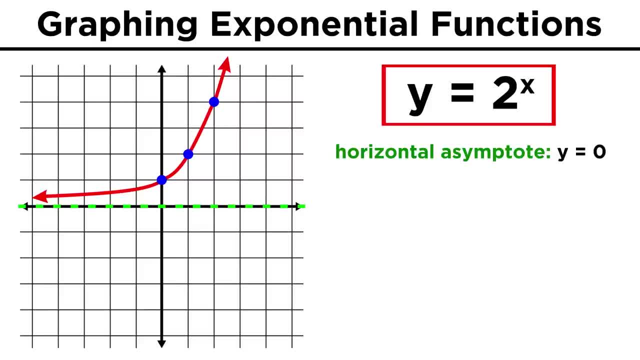 Once again, two to the X looks like this: It has a horizontal asymptote in the X axis and the function will always be positive because there is no exponent that two can be raised to in order to get a negative number. Negative exponents, as we recall, still produce positive values as two to the negative one. 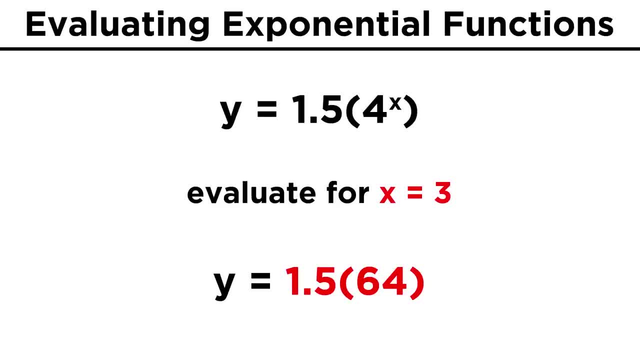 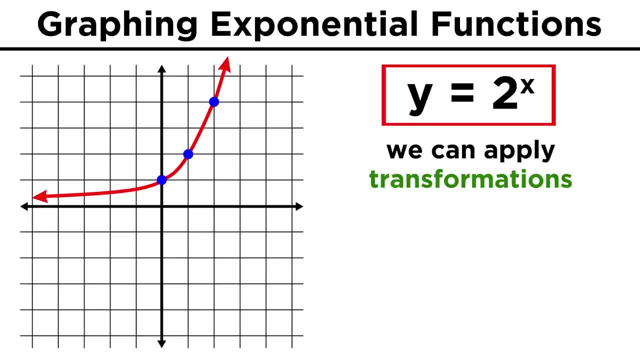 we just cube four to get sixty-four and then multiply by one point five to get ninety-six. Graphing can be a little trickier, but as long as we know what the basics look like, we can apply transformations just like we did for parabolas. 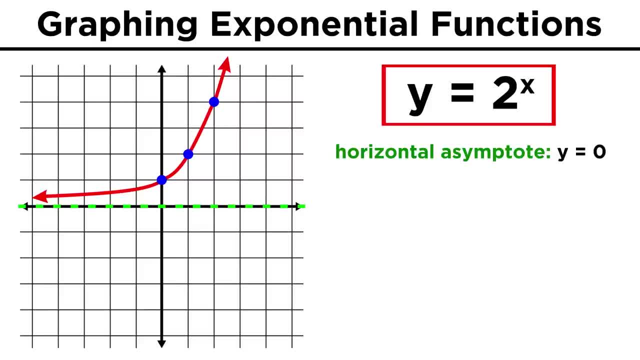 Once again, two to the X looks like this: It has a horizontal asymptote in the X axis and the function will always be positive because there is no exponent that two can be raised to in order to get a negative number. Negative exponents, as we recall, still produce positive values as two to the negative one. 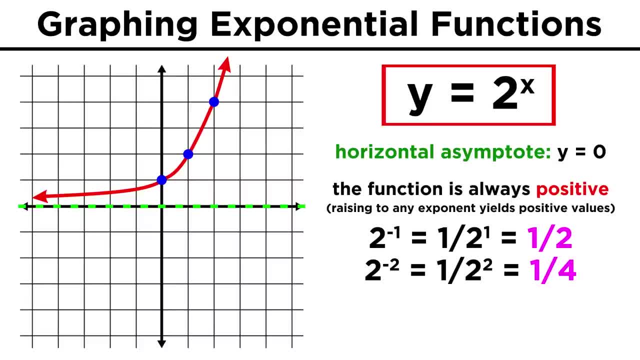 is just one half, Two to the negative, two is one over two squared, or one fourth and so on, getting closer to zero as the exponent increases in the negative one. That's why we call it a positive exponent In the positive direction. as the exponent increases, the function approaches positive. 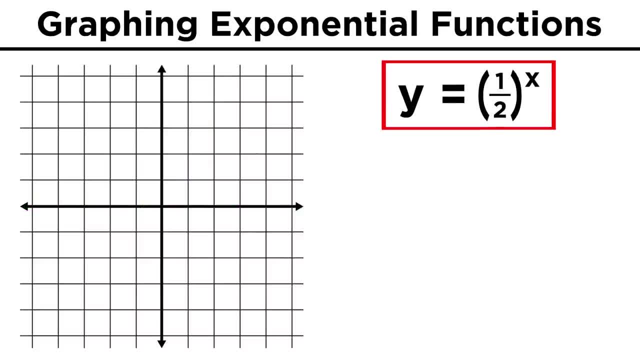 infinity. Now let's look at one half to the X. Now, as the exponent increases, the function approaches zero. so there is again a horizontal asymptote in the X axis: As the exponent becomes increasingly negative, the function approaches positive infinity. This is actually the same as two to the negative. 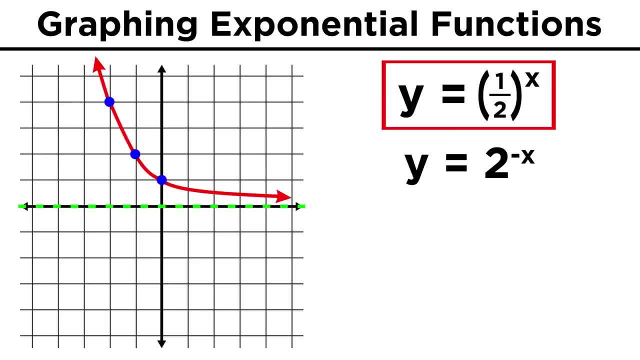 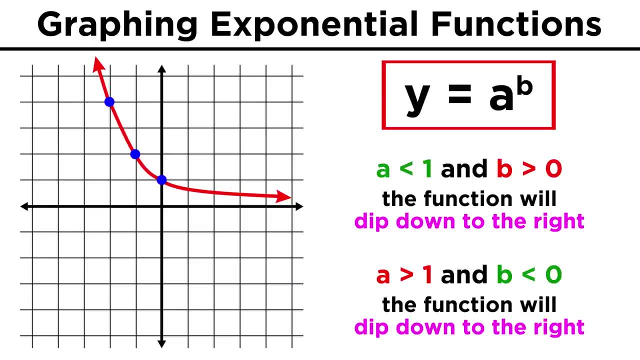 So negative one, two to the negative. one is one half to the negative X, because to get rid of the negative sign on the exponent we invert the base, which would give us one half to the X. This means that for exponential functions, if the base is less than one and the exponent 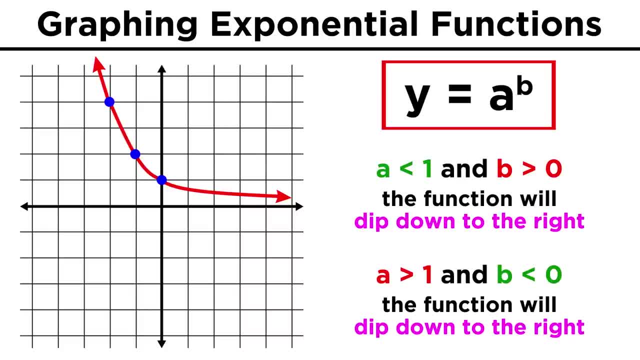 is positive, or if the base is greater than one and the exponent is negative, the function dips down to the right. like this: When the exponent is positive and the base is less than one, the function comes down to the right. or if the base is less than one and the exponent is negative, the function will rise up to. 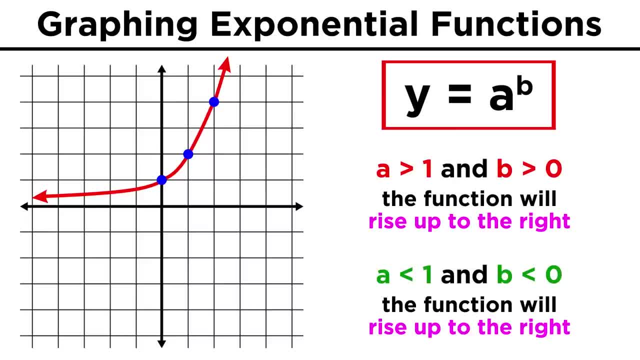 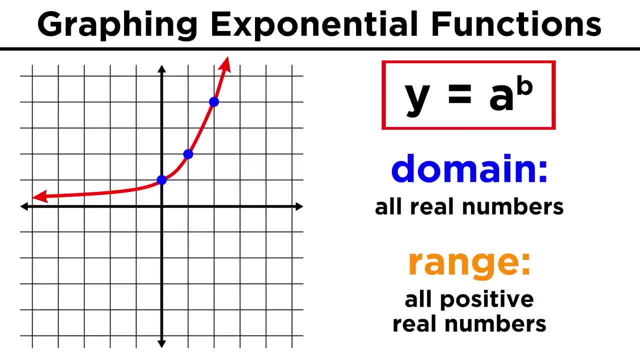 the right, like the previous example, But in both cases the domain is all real numbers and the range is all real numbers greater than zero. As we said, we can graph alterations of this basic form by applying transformations. Adding or subtracting a number here will generate a vertical shift. 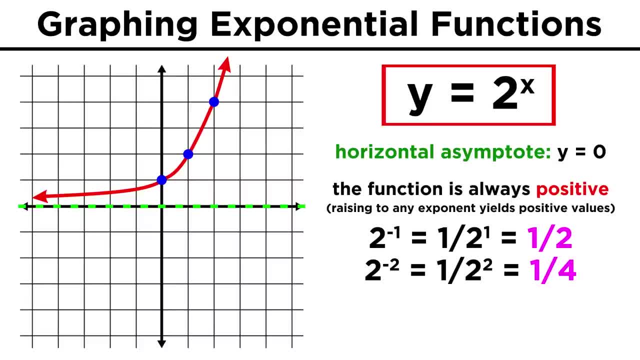 is just one half, Two to the negative, two is one over two squared, or one fourth and so on, getting closer to zero as the exponent increases in the negative one. That's why we call it a positive exponent In the positive direction. as the exponent increases, the function approaches positive. 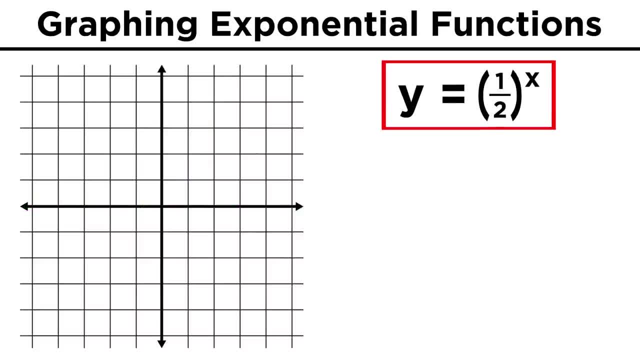 infinity. Now let's look at one half to the X. Now, as the exponent increases, the function approaches zero. so there is again a horizontal asymptote in the X axis: As the exponent becomes increasingly negative, the function approaches positive infinity. This is actually the same as two to the negative. 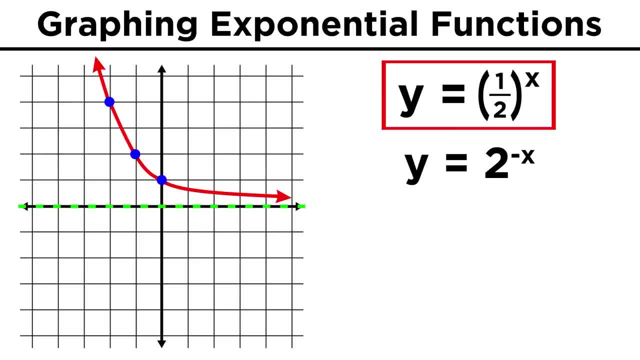 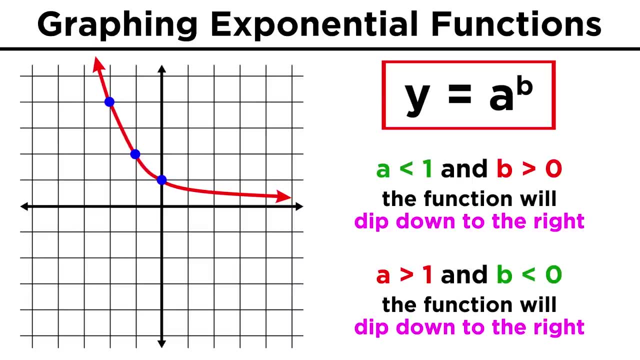 So negative one has two half to the negative X because to get rid of the negative sign on the exponent we invert the base, which would give us one half to the X. This means that for exponential functions if the base is less than one and the exponent 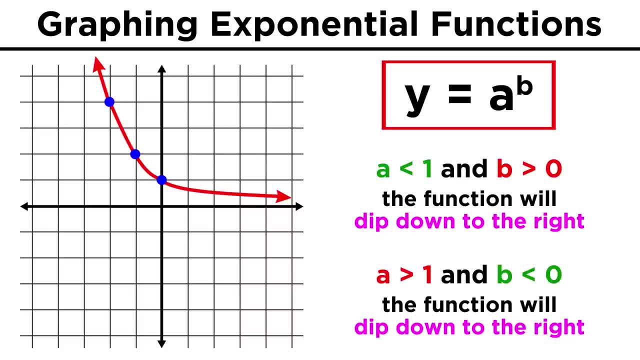 is positive, or if the base is greater than one and the exponent is negative, the function dips down to the right, like this: 1 and the exponent is positive, or if the base is less than 1 and the exponent is negative, the function will rise up to the right, like the previous example. 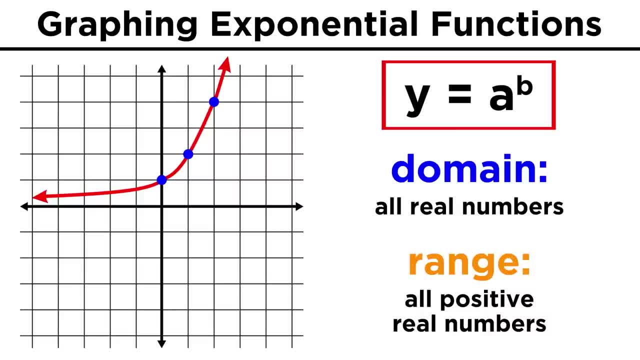 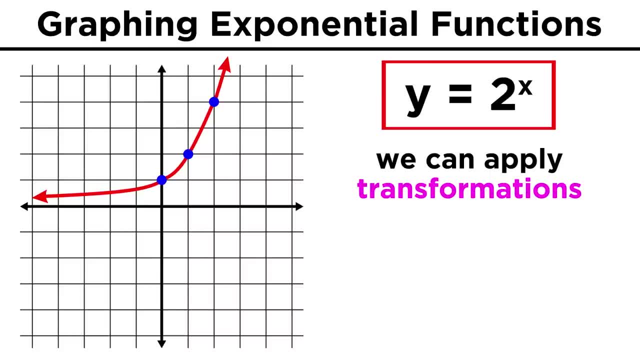 But in both cases the domain is all real numbers and the range is all real numbers greater than zero. As we said, we can graph alterations of this basic form by applying transformations. Adding or subtracting a number here will generate a vertical shift. 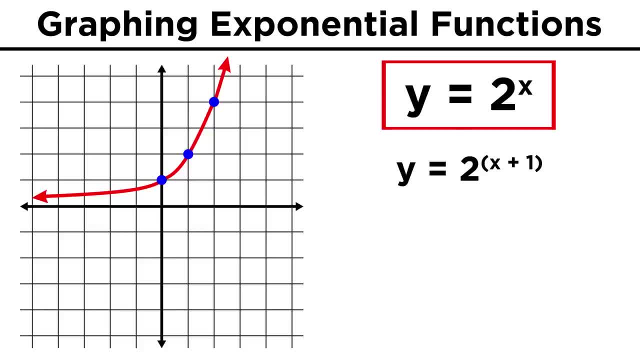 Adding or subtracting a number from the variable term right here, like two, to the X plus one, will produce a horizontal shift. If we put a negative sign here, we get a reflection across the X axis, since all the positive values become negative values. 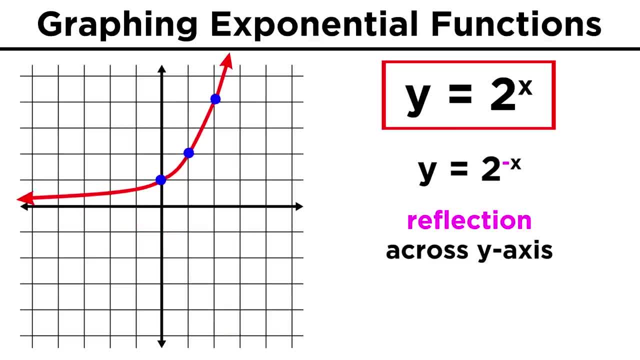 If instead we put the negative sign here before the variable, we get a reflection across the Y axis, Just as we saw earlier, with two to the negative X. And lastly, a coefficient here or here will produce vertical stretching and horizontal stretching respectively.